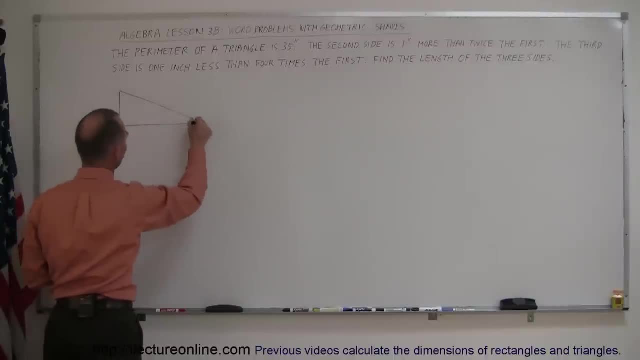 draw a triangle Could be any shape triangle like so, and I have three sides. So let's call this the first side, let's call this the second side and let's call this the third side. Now they tell us that the perimeter of this triangle, 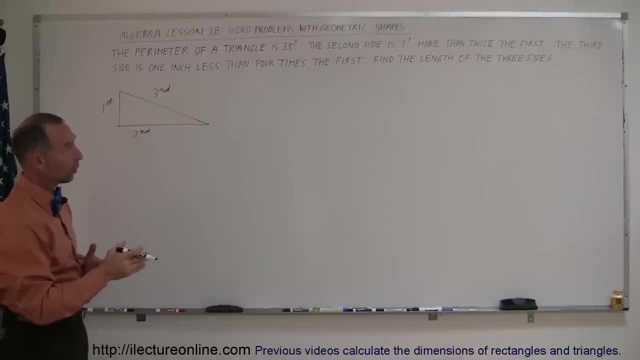 triangle is 35 inches, And then they tell us that the second side is one inch more than twice the first. The third side is one inch less than four times the first. Find the length of the three sides. So let's start off by assuming that the first is the smallest one. That seems to be the 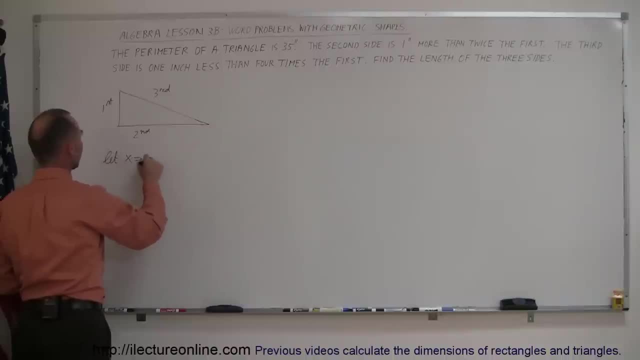 indication here. So let x equal the length of the first side, So length of first side. All right, then how would you express the second side? And it says here that the second side is one inch more than twice the first. So twice the first that's 2x, and one inch more would be plus one, So that's. 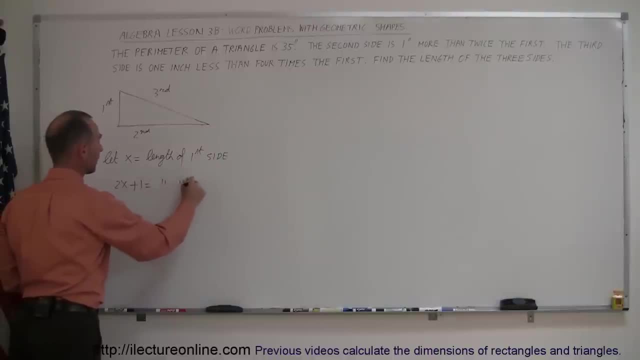 twice the first plus one equals the length of the second side. Now the third side, It is one inch less than four times the first. So four times x, that would be four times the first and then one inch less. we subtract one from that so that equals the length of the second side, So that 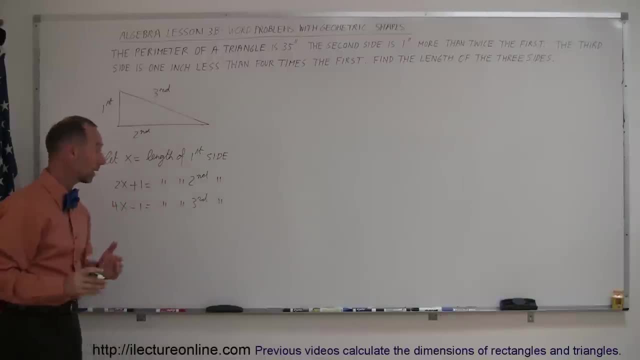 equals the length of the third side. All right, so now we have the length of the first side, the second side and the third side expressed in terms of x. Now we can go ahead and solve the problem. It says here that the triangle is 35 inches. That means the length of the first side plus the length 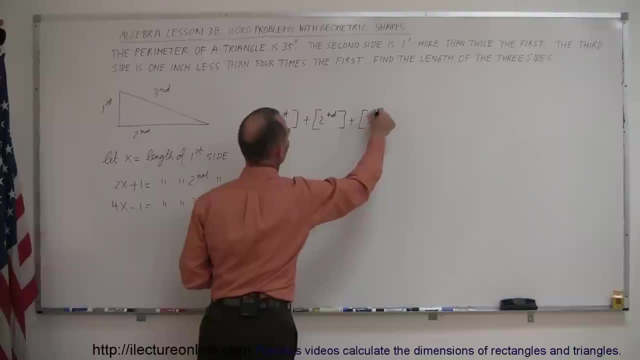 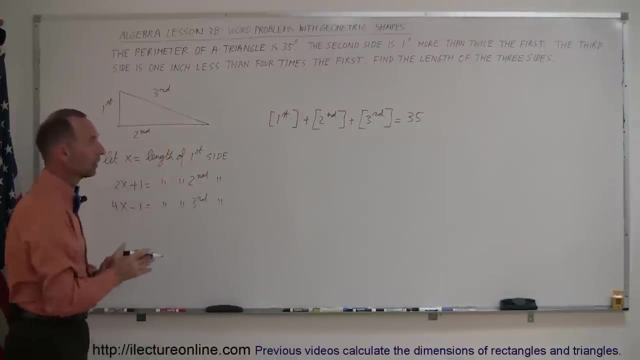 of the second side plus the length of the third side equals the perimeter, or 35 inches. Okay, so that's kind of a graphical way to represent the length of the first side. Now we're going to plug in the meaning of each of those in terms of x. So x is the length of the. 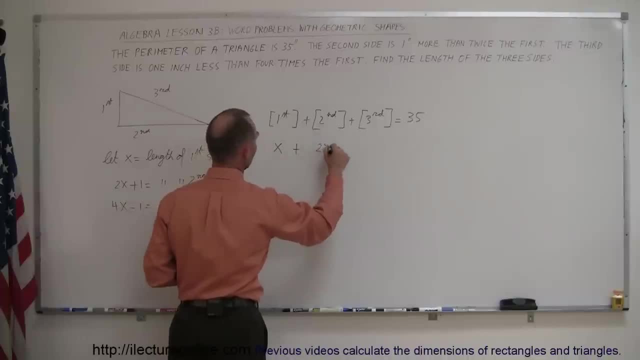 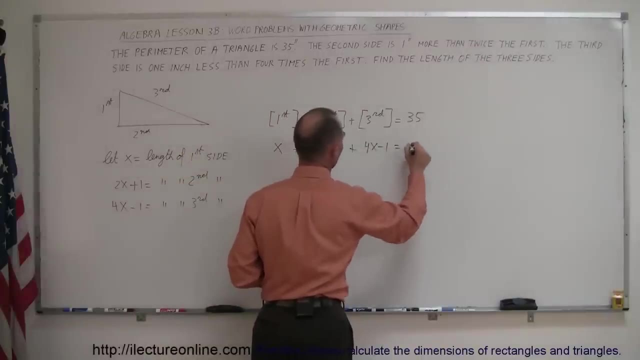 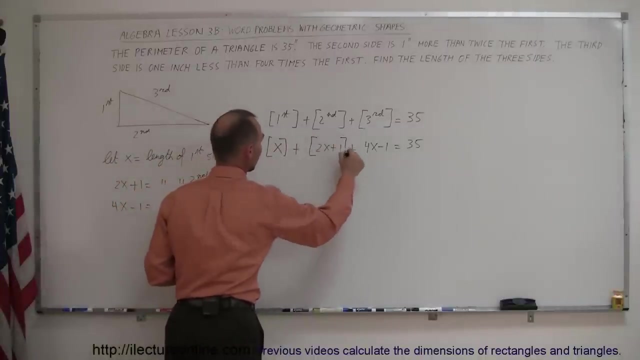 first side, plus 2x plus one the length of the second side, plus 4x minus one length of the third side, and that adds up to the perimeter. So always get the feel here that we know what we're doing with substituting into each of the sides what the sides are represented as.